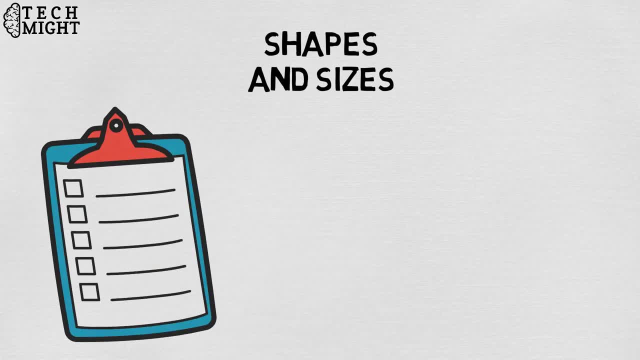 efficiently carry out the task for which they are designed. All robots vary in design, functionality and degree of autonomy. From the 0.2 millimeter long Robobee to the 200 meter long robotic shipping vessel Vineskip, robots are emerging to carry out tasks that humans simply can't. 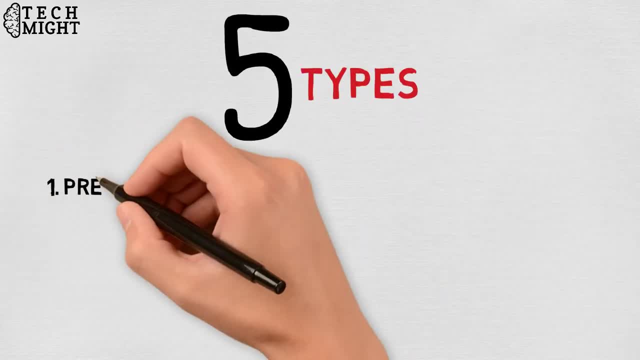 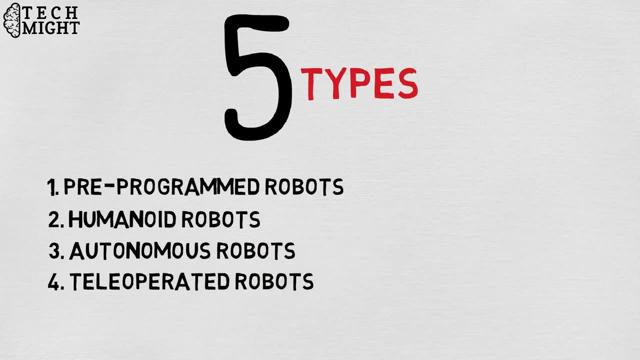 Generally, there are five types of robots: 1. Pre-programmed robots. 2. Humanoid robots. 3. Autonomous robots. 4. Tele-operated robots. 5. Augmenting robots. 4. Autonomous robots 5.. 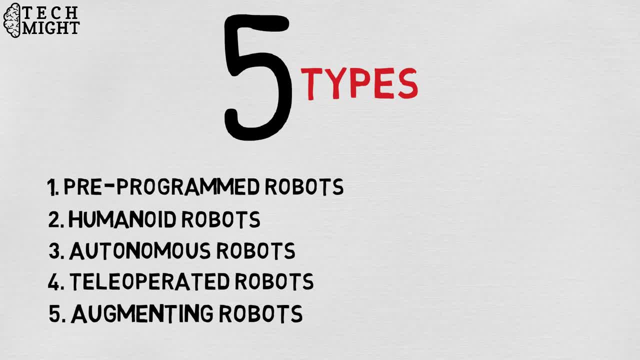 Tele-operated robots, 5. Augmenting robots, 5. Tele-operated robots, 5. Augmenting robots, 5. Augmenting robots. Let's discuss these types in detail. Pre-programmed robots- Pre-programmed robots. 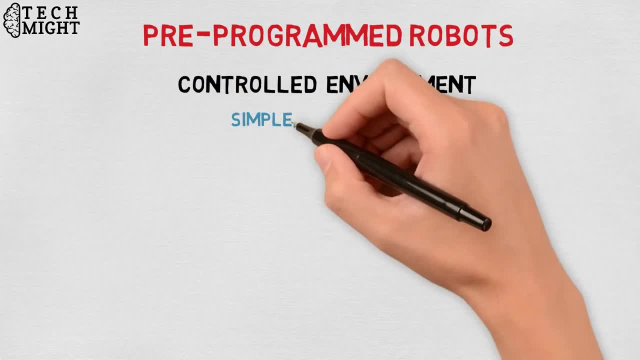 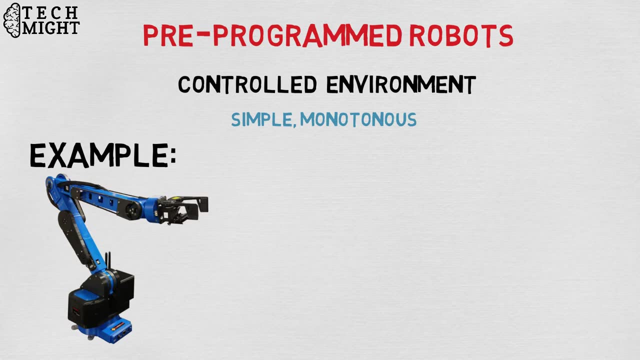 operate in a controlled environment where they do simple, monotonous tasks. An example of a pre-programmed robot would be a mechanical arm on an automotive assembly line. The arm serves one function: to weld a door on, to insert a certain part into the engine, etc. and its job is to 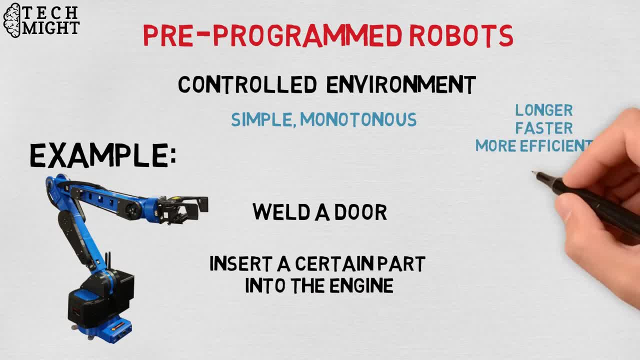 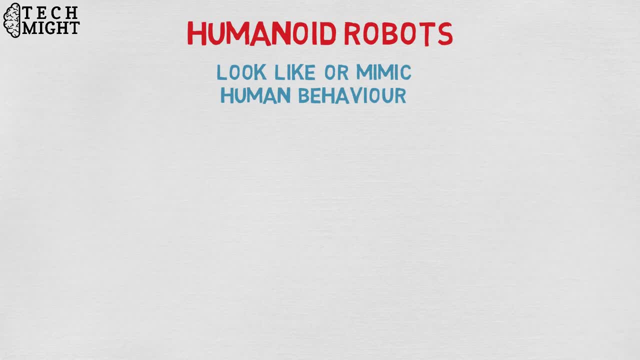 perform that task longer, faster and more efficiently than a human Humanoid robots. Humanoid robots are robots that look like and or mimic human behavior. These robots usually perform human-like activities like running, jumping and carrying objects, and are sometimes 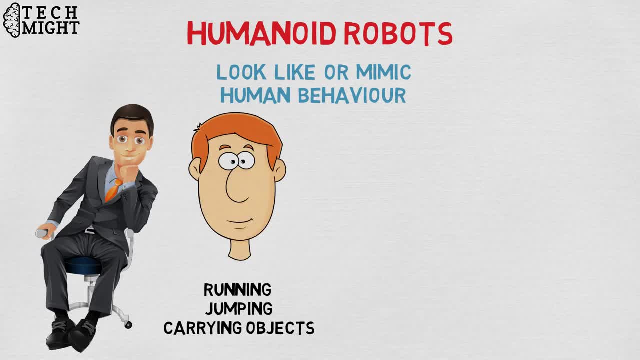 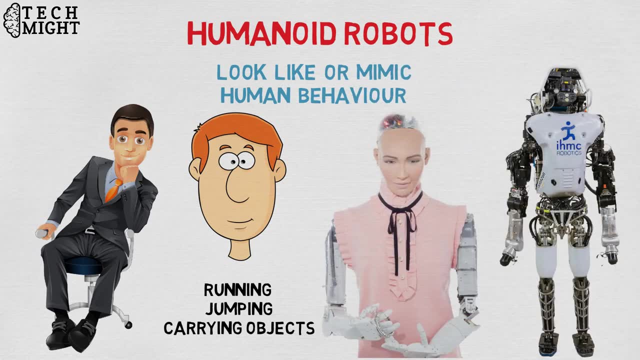 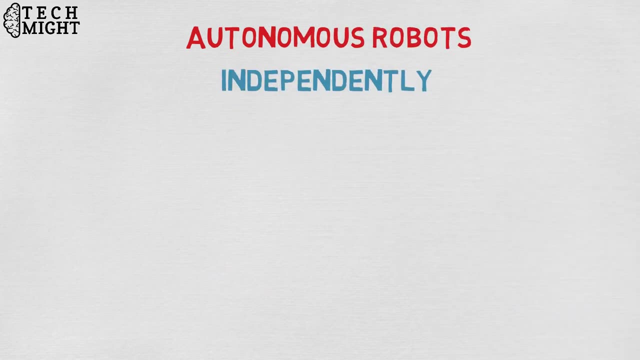 designed to look like us, even having human faces and expressions. Two of the most prominent examples of humanoid robots are Hanson Robotics' Sophia and Boston Dynamics Atlas Autonomous robots. Autonomous robots operate independently of human operators. These robots are usually designed to carry out tasks in open environments that do not require human supervision. They are 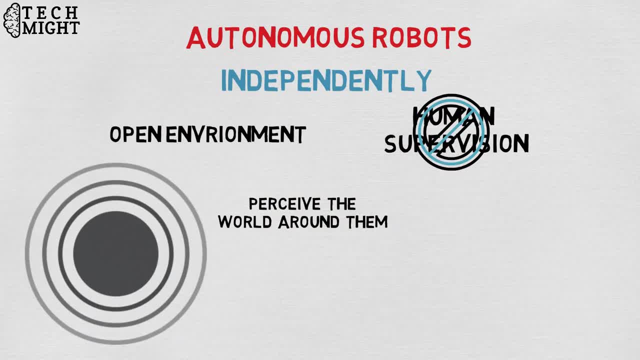 quite unique because they use sensors to perceive the world around them and then employ decision-making structures, usually a computer, to take the optimal next step based on their data and mission. An example of an autonomous robot would be the Roomba Vacuum Cleaner, which uses sensors to roam. 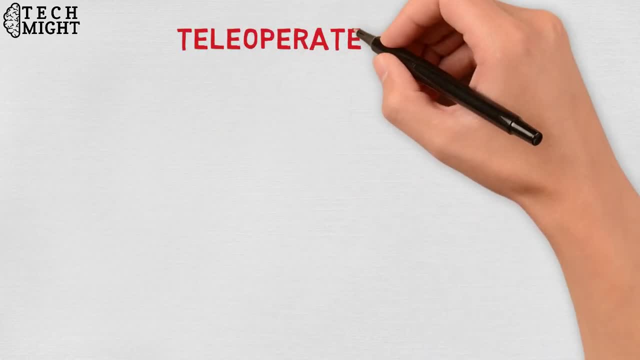 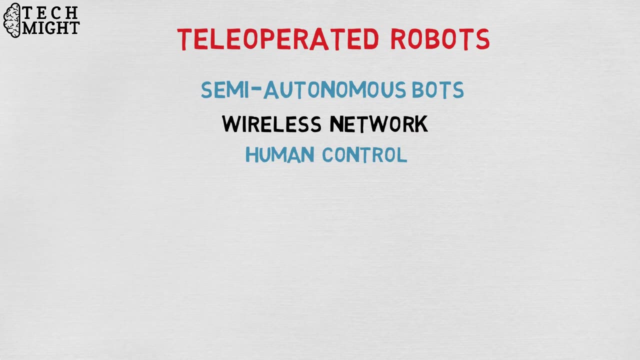 freely throughout a home. Teleoperated robots. Teleoperated robots are semi-autonomous bots that use a wireless network to enable human communication. Teleoperated robots are semi-autonomous and can control from a safe distance. These robots usually work in extreme geographical.